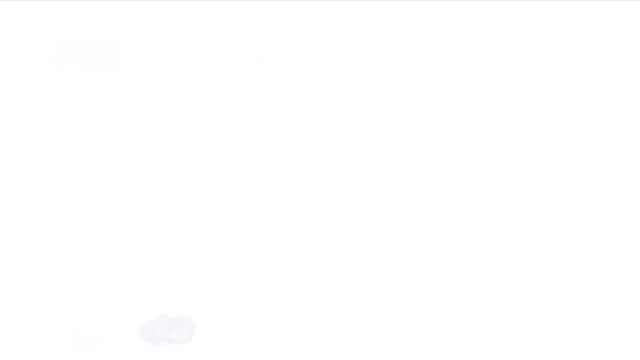 thing correctly. Now, when acids react with metal carbonates, the reaction's pretty similar: They still form a salt and water, but we also get carbon dioxide. So if we took nitric acid and combined it with calcium carbonate, then it, just like before, would form a salt and water, but we 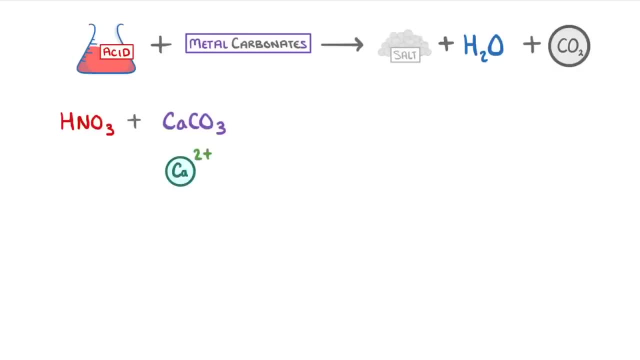 still have to balance it. So what we'd do is take the positive calcium ion from our base and combine it with the negative nitrate ions from the acid, But because the nitrate only has a 1 minus charge, while the calcium's 2 plus, we'd 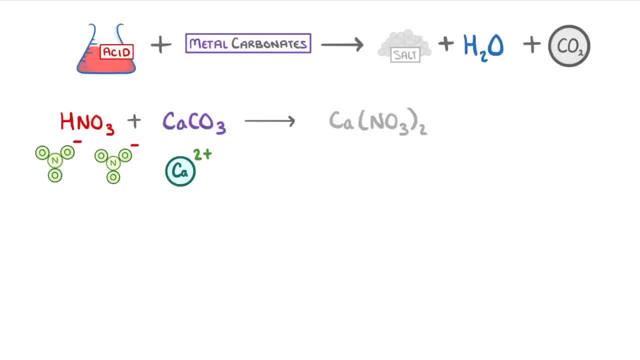 need two of them to form calcium nitrate, which would be our salt, And then we'd also get water and carbon dioxide and have to check it's balanced. Now, all of the salts that we've covered so far have been soluble in water, meaning they 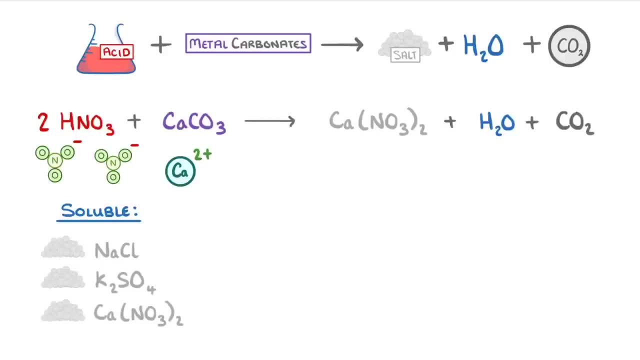 dissolve. So if we want to make a soluble salt, all we need to do is react an acid with an insoluble base, like a metal oxide, hydroxide or carbonate. In practice, though, to actually carry out this reaction, there are a few different steps that you need to know. First, you place some dilute acid. 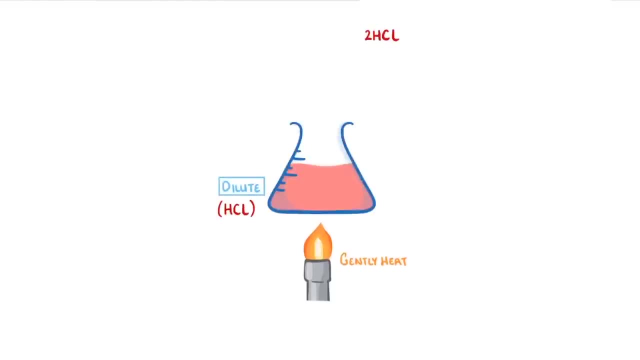 for example hydrochloric acid in a beaker and gently heat it with a Bunsen burner. Then you keep adding insoluble base, for example copper oxide, a little bit at a time. At first it will keep disappearing as it reacts to form aqueous copper chloride and water. 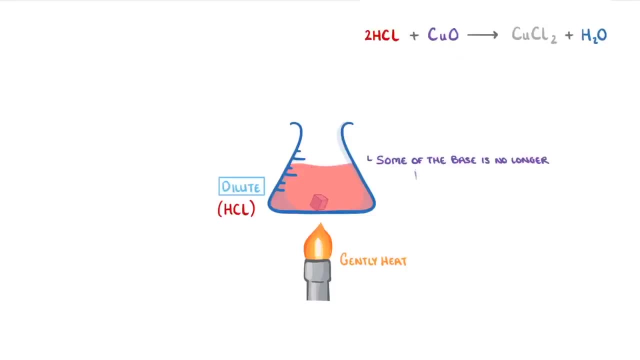 but then, as you add more, you'll see that some of the base is no longer disappearing. So at this point we know that the base must be in excess and we'll have neutralised all of the acid. The next step is to filter out all of this excess copper oxide. and then add a little bit of hydrochloric acid. So at this point we know that the base must be in excess and we'll have neutralised all of the acid. So at this point we know that the base must be in excess and we'll have neutralised all of the acid. 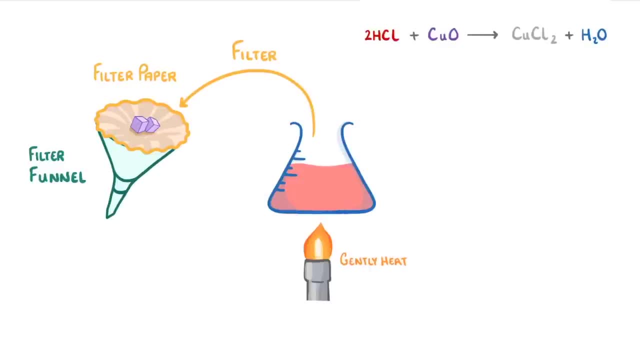 Using filter paper and a filter funnel, and what we have left should be the dissolved form of our soluble salt, in this case copper chloride. In order to get pure solid crystals of copper chloride, though, we'd need to gently heat up our now filtered solution and evaporate off some of the water.